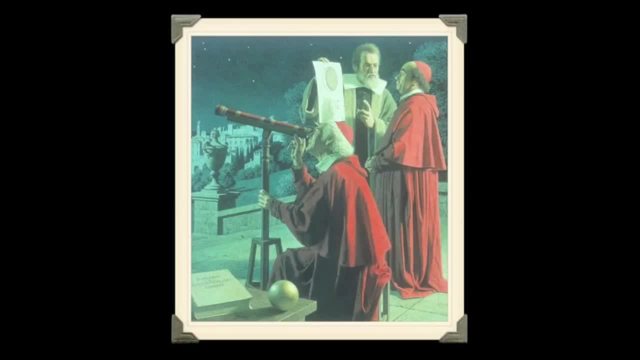 go through phases, just like the moon. He also noted that the planet Jupiter had several moons of its own. In addition, Galileo was the first to see that there were actually spots on the surface of the sun that moved as days went by. 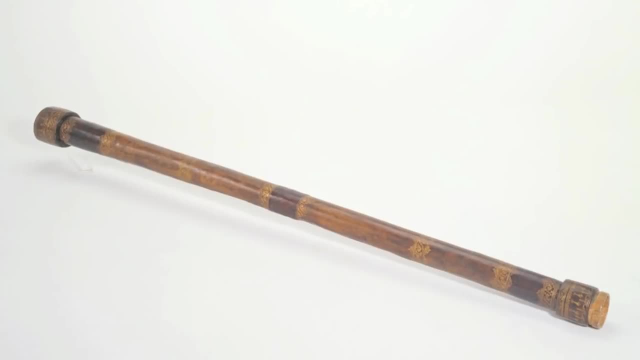 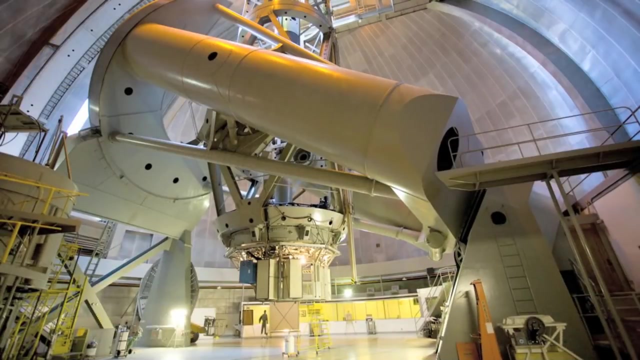 Telescopes have improved quite a bit throughout history. They've grown larger and more powerful. Modern observatories today have massive telescopes with huge glass lenses that allow us to peer to the depths of the universe. We even have a major telescope that's currently 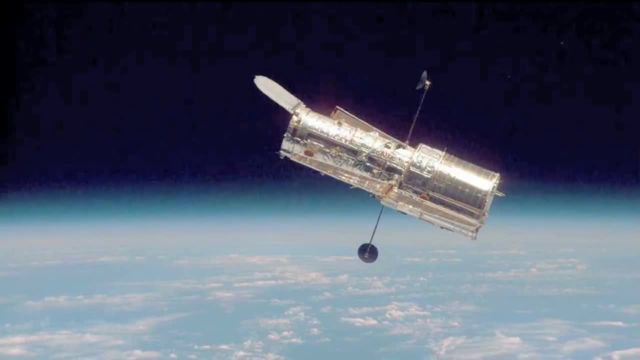 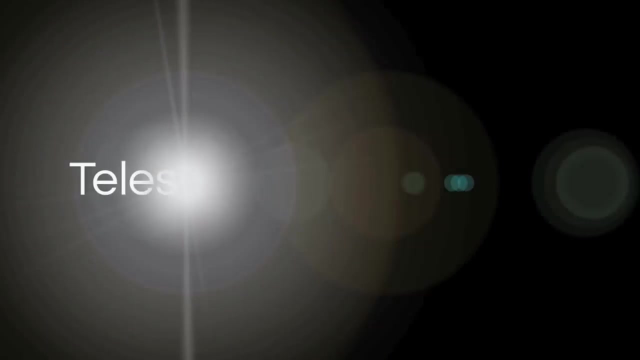 orbiting the Earth, which is able to see the very beginning of the universe, But we'll talk more about that later on. So why is it that these telescopes are just so important to our understanding of the universe? What is it that a telescope does? Well, it's pretty simple, actually: Telescopes collect. 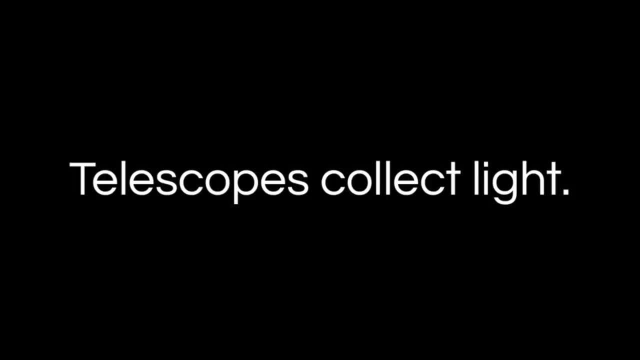 light. When we point a telescope up at the sky, no matter how large or small it may be, what it's doing is collecting light that's flying throughout space. It's amazing how much we can learn about the universe just by studying this light- In fact, that's. 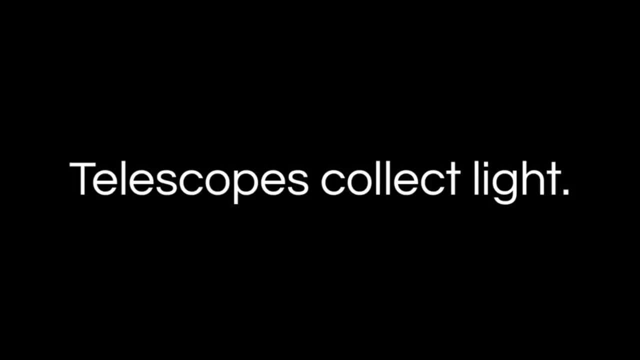 actually what astronomy is? It ends up being the study of all of the light flying around in the universe. It's amazing what we can gain by studying this light, But this brings up another question: What exactly is light, then? Well, that also can be answered with this simple response: Light is energy, But again, 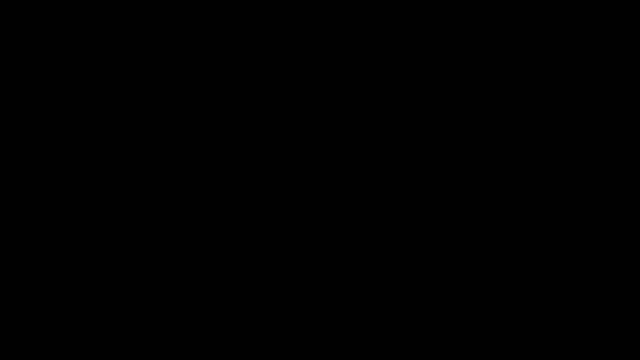 this leads us to yet another misunderstanding. What exactly is energy? Well, if you look it up in the dictionary, energy is defined as the ability to do work, the ability to have an impact on something. What makes it such a tricky concept, though, is that there's 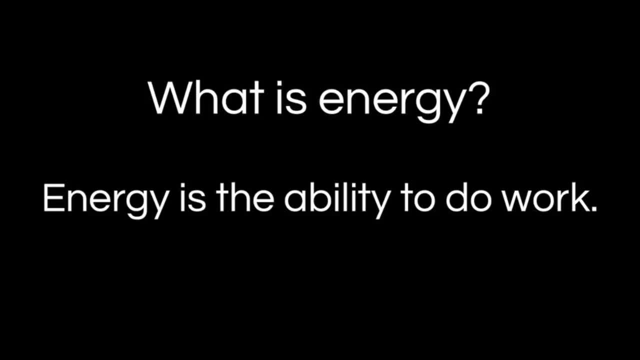 many different kinds of energy that are very unique and very important to our understanding of the universe, And that's exactly what we're going to talk about today. We're going to be looking at the different types of energy that are very different from each other: Energy- 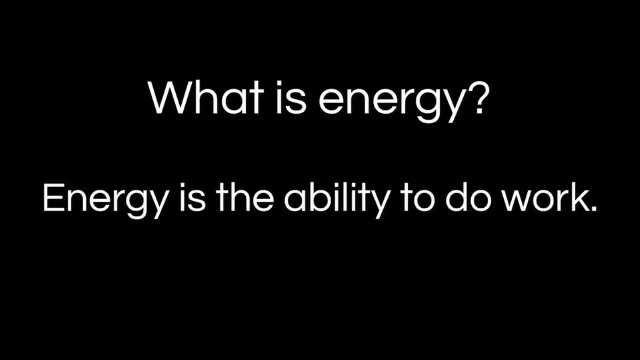 includes mechanical energy, thermal energy, electrical energy, nuclear energy, light and heat, amongst others, And all of it can be actively working in the form of kinetic energy, Or it could be stored up for future use in the form of potential energy, It turns out. 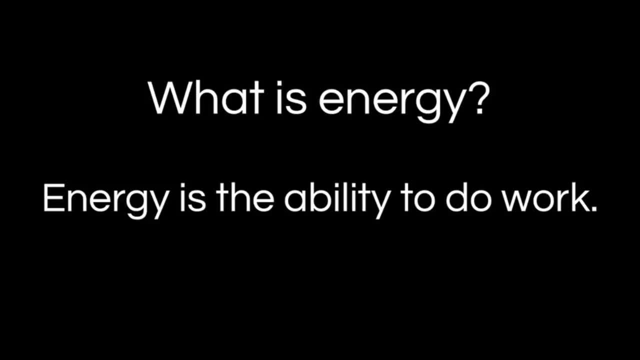 that in the study of astronomy, the most important type of energy is light and heat, And this is shown in this example, in its different types, on a diagram known as the electromagnetic spectrum. let's take a look at a short video from nasa which explains what the electromagnetic spectrum is and how exactly it. 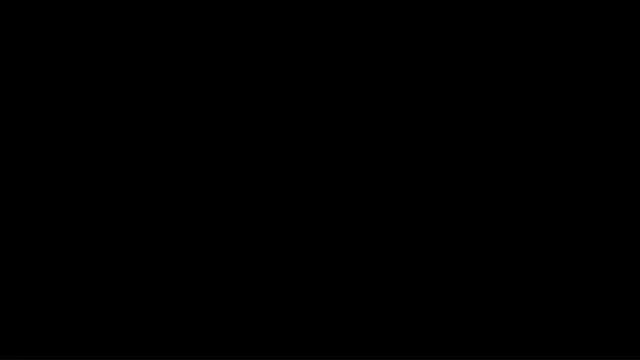 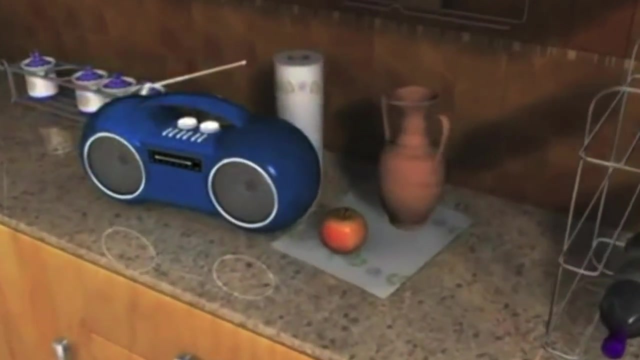 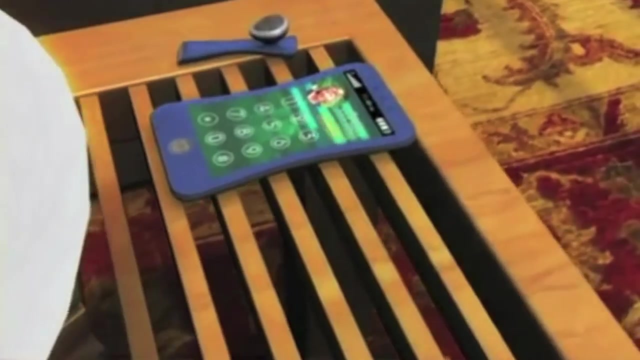 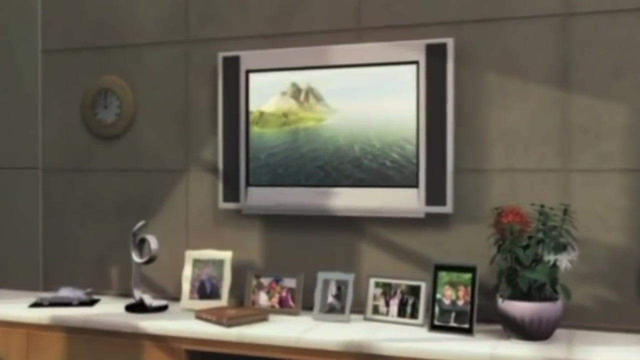 works, something surrounds you, bombards you, some of which you can't see, touch or even feel every day, everywhere you go. it is odorless and tasteless, yet you use it and depend on it every hour of every day. without it, the world you know could not exist. what is it? electromagnetic radiation? 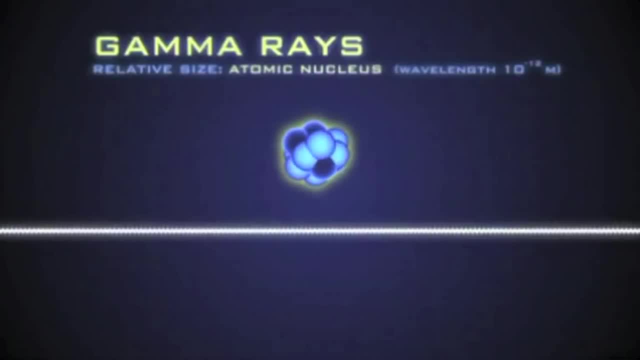 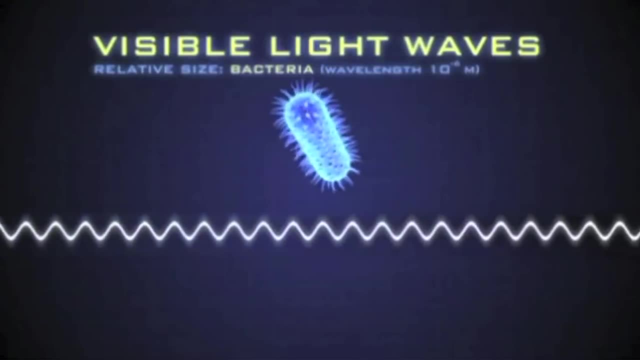 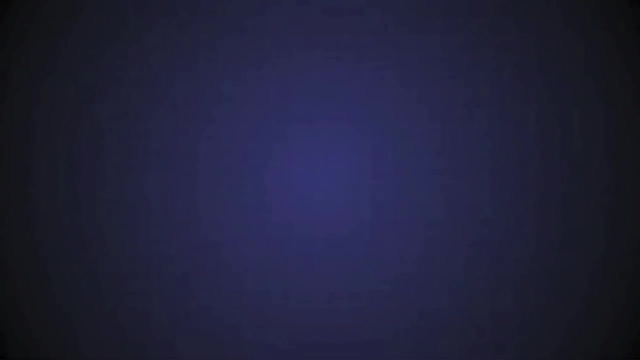 these waves spread across a spectrum from very short gamma rays to x-rays, ultraviolet rays, visible light waves, even longer infrared waves, microwaves to Radio waves which can measure longer than a mountain range. This spectrum is the foundation of the information age and of our modern world. 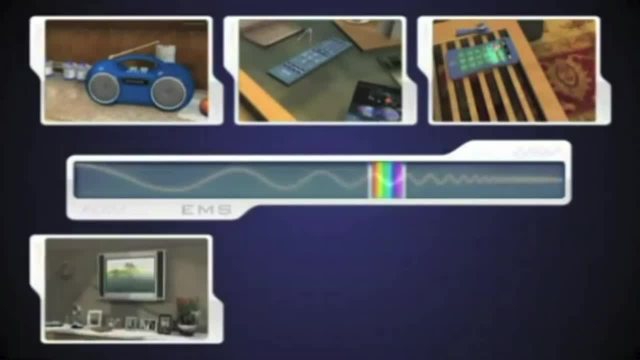 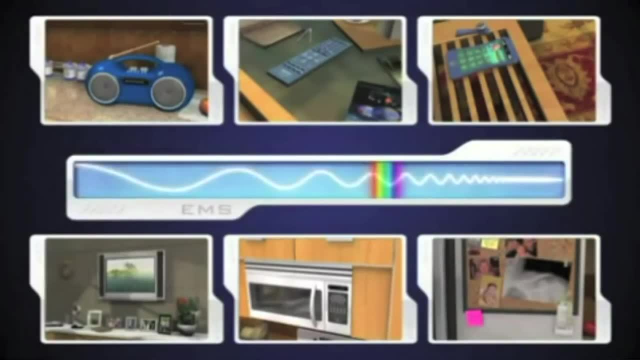 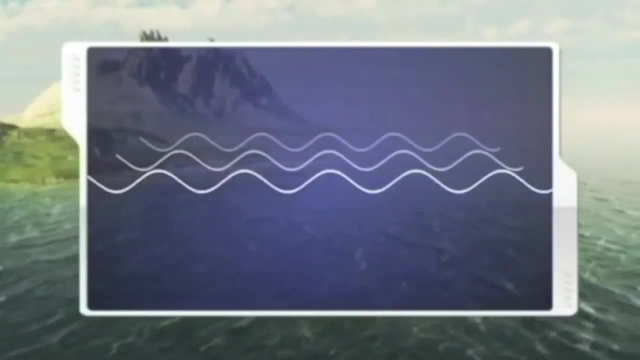 Your radio remote control, text message, television, microwave oven, even a doctor's x-ray, all depend on waves within the electromagnetic spectrum. Electromagnetic waves, or EM waves, are similar to ocean waves in that both are energy waves. 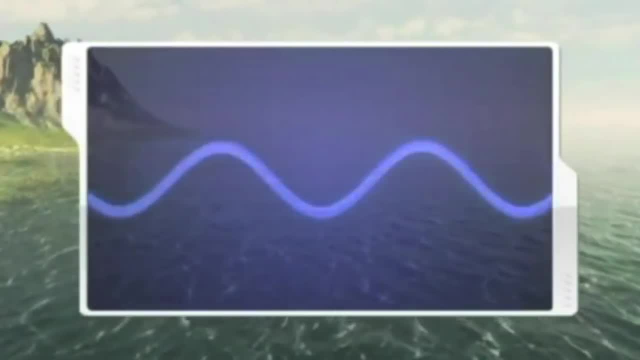 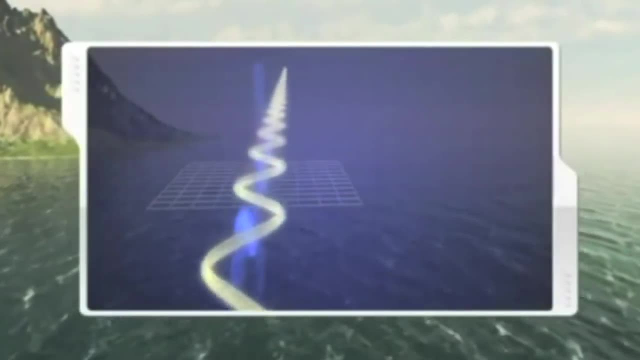 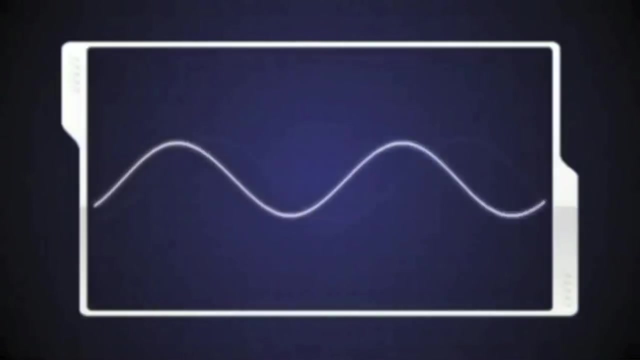 They transmit energy. EM waves are produced by the vibration of charged particles and have electrical and magnetic properties, But unlike ocean waves that require water, EM waves travel through the vacuum of space at the constant speed of light. EM waves have crests and troughs. like ocean waves. 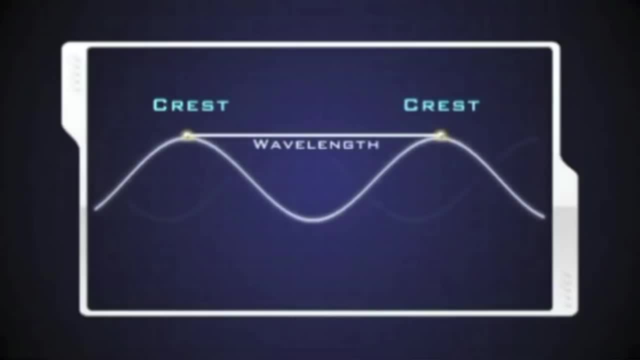 The distance between crests is the wavelength. While some EM wavelengths are very long and are measured in meters, many are tiny and are measured in billions. The number of these crests that pass a given point within one second is described as the frequency of the wave. 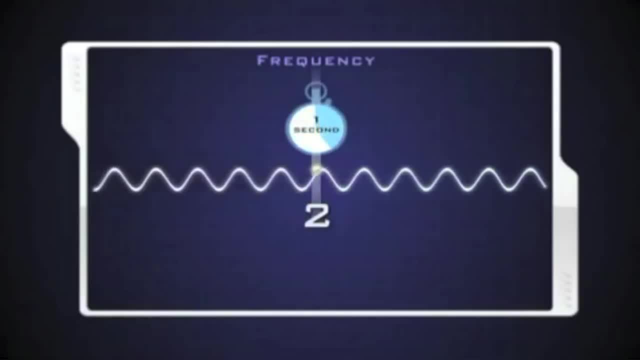 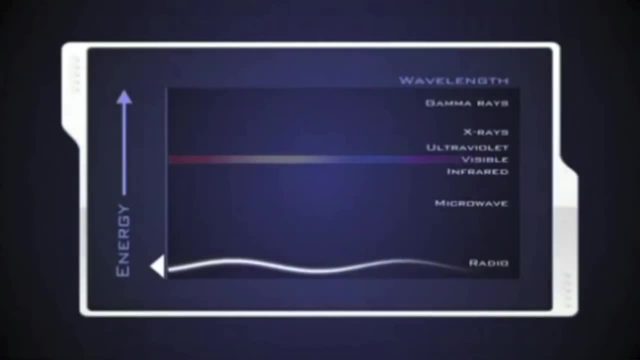 One wave or cycle per second is called a hertz Long. EM waves, such as radio waves, have the lowest frequency and carry less energy. Adding energy increases the frequency of the wave and makes the wavelength shorter. Gamma rays are the shortest, highest energy waves in the spectrum. 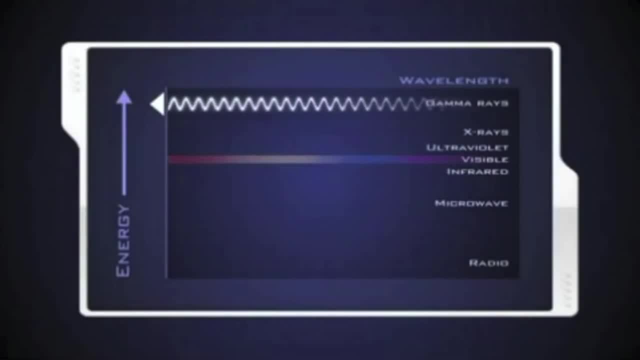 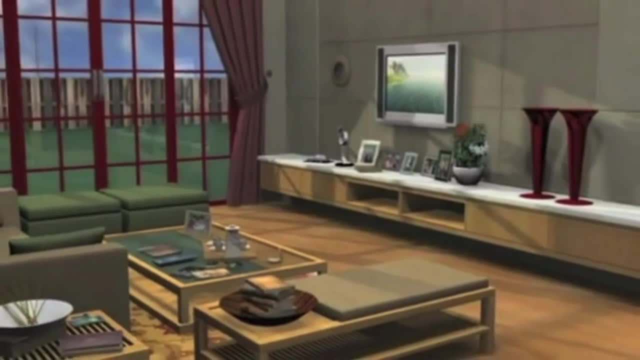 The frequency of the wave varies depending on the frequency of the wave. The frequency of the wave varies depending on the frequency of the wave. The frequency of the wave varies depending on the frequency of the wave. So, as you sit watching TV, not only are there visible light waves from the TV striking your eyes, 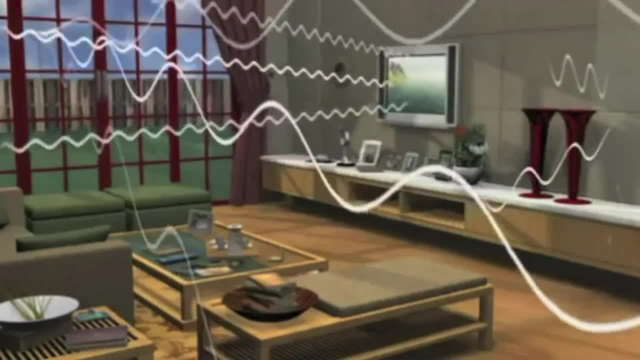 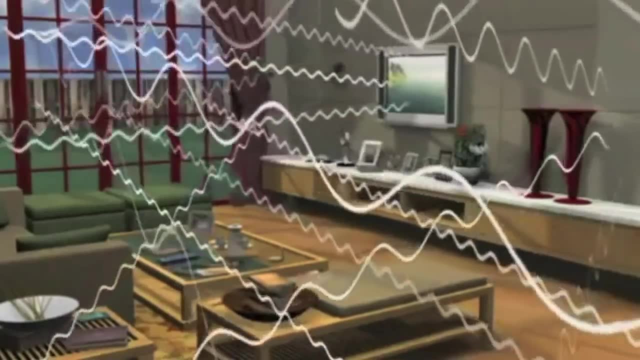 but also radio waves transmitting from a nearby station and microwaves carrying cell phone calls and text messages, and waves from your neighbor's Wi-Fi and GPS units in the cars driving by. There is a chaos of waves from all across the spectrum passing through your room right now. 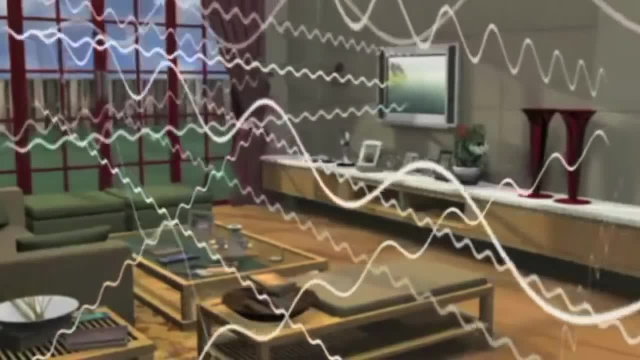 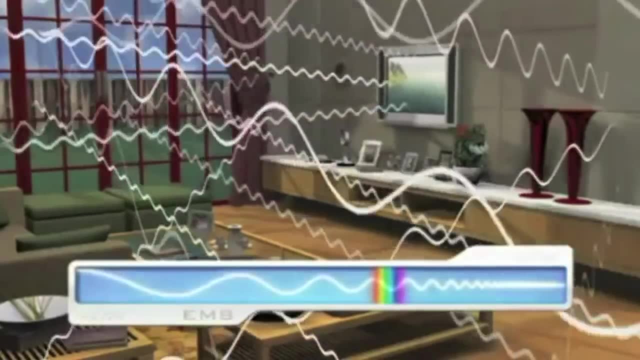 With all these waves around you, how can you possibly watch your TV show? Similar to tuning a radio to a specific radio station, our eyes are tuned to a specific region of the EM spectrum and can detect energy with wavelengths from 400 to 700 nanometers. 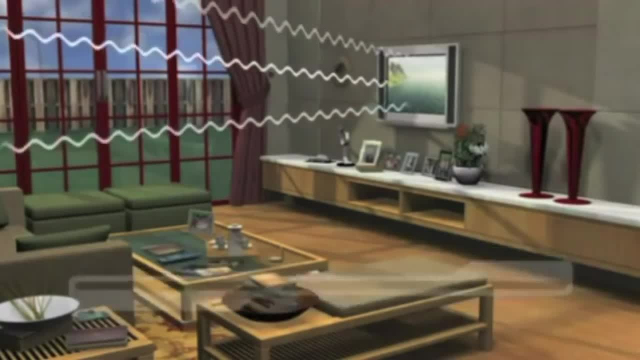 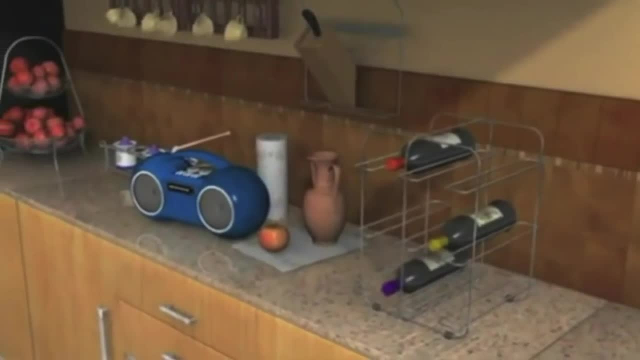 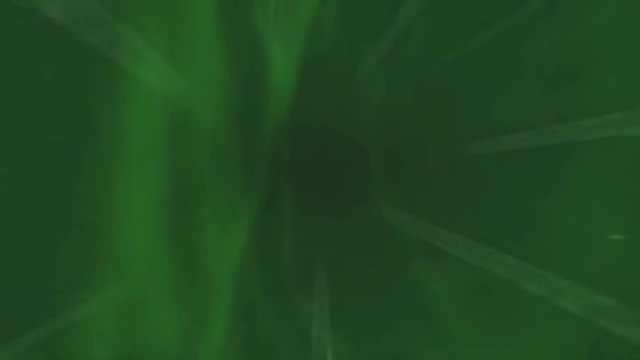 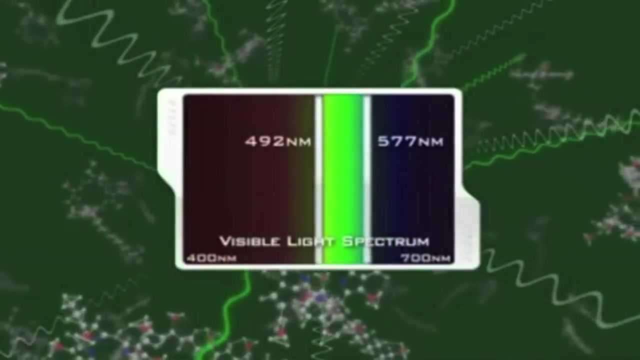 the visible light region of the spectrum. Objects appear to have color because EM waves interact with their molecules. Some wavelengths in the visible spectrum are reflected and other wavelengths are absorbed. This leaf looks green because EM waves interact with their molecules. Waves between 492 and 577 nanometers in length are reflected. 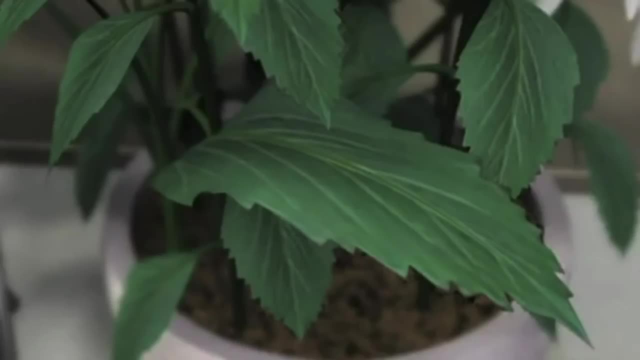 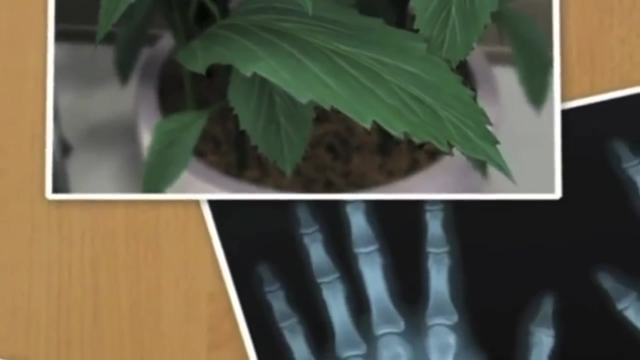 and our eye interprets this as the leaf being green. Our eyes see the leaf as green, but cannot tell us anything about how the leaf reflects ultraviolet, microwave or infrared waves. To learn more about the world around us, scientists and engineers have devised ways to enable us to see beyond that sliver of the EM spectrum. 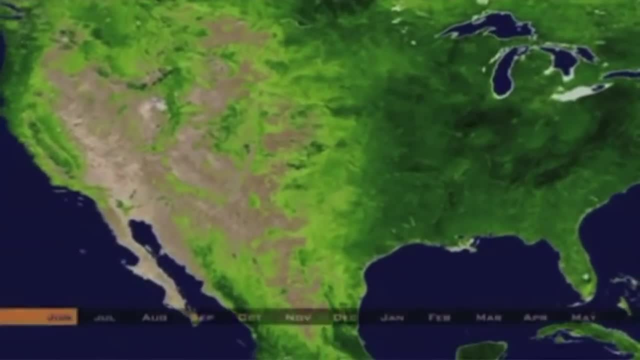 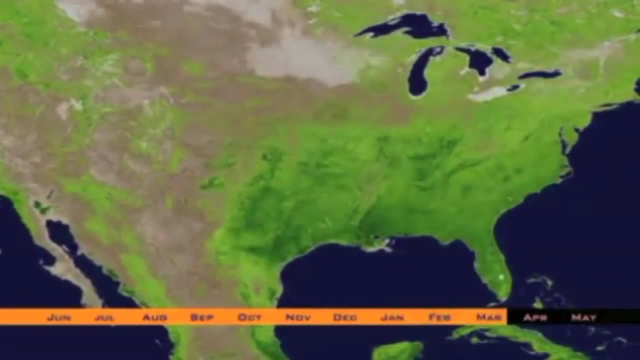 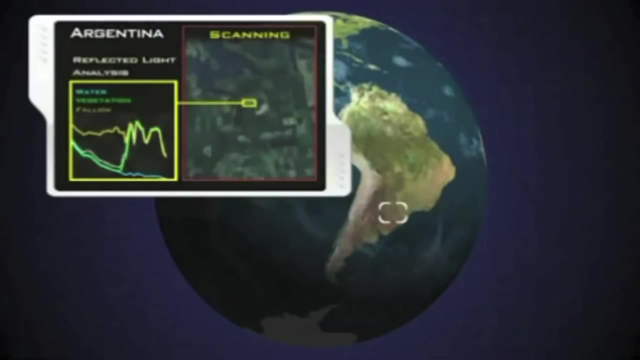 called visible light. Data from multiple wavelengths help scientists study all kinds of amazing phenomena on Earth, from seasonal change to specific habitats. Everything around us emits, reflects and absorbs EM radiation differently based on its composition. A graph showing these interactions across a region of the EM spectrum is called a spectral signature. 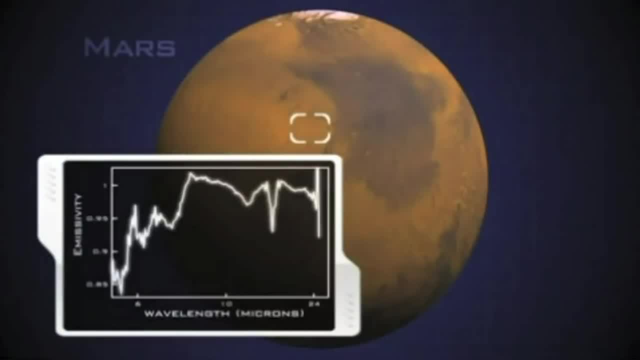 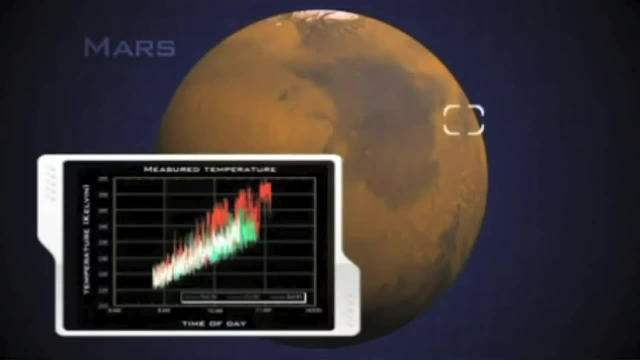 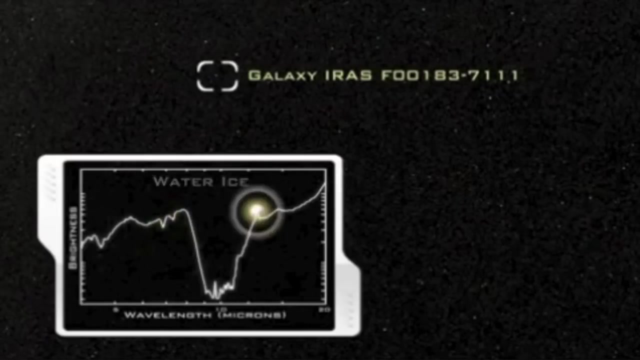 Characteristic patterns like fingerprints within the spectra allow astronomers to identify an object's chemical composition and to determine such physical properties as temperature and density. NASA's Spitzer Space Telescope observed the presence of water and organic molecules in a galaxy 3.2 billion light years away. 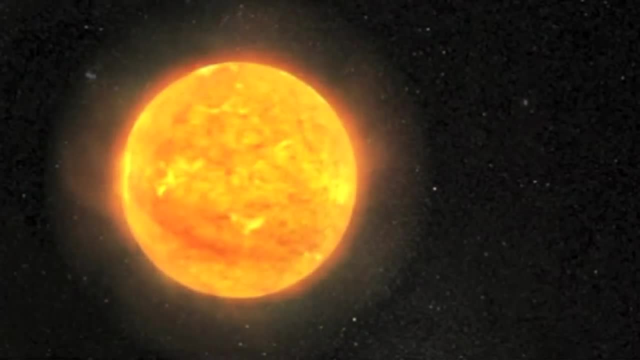 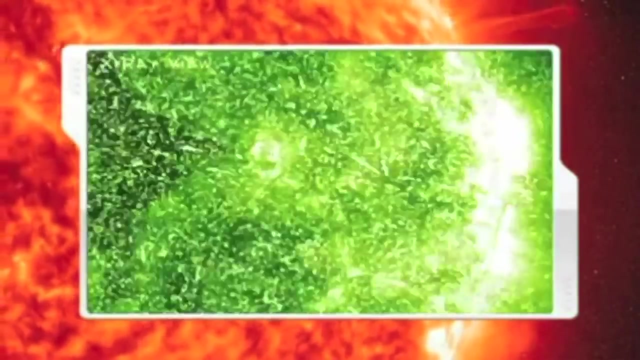 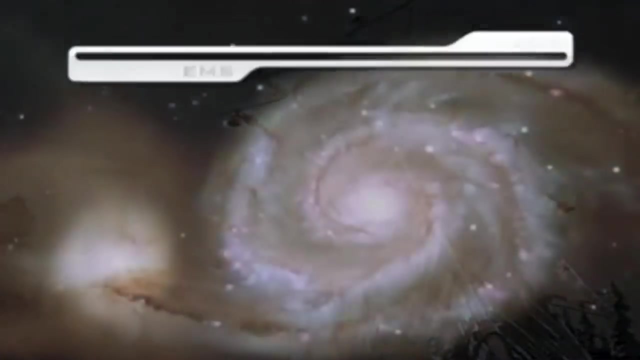 Viewing our sun in multiple wavelengths with the SOHO satellite allows scientists to study and understand sunspots that are associated with solar flares and eruptions harmful to satellites, Astronauts and communications here on Earth. We are constantly learning more about our world and universe. 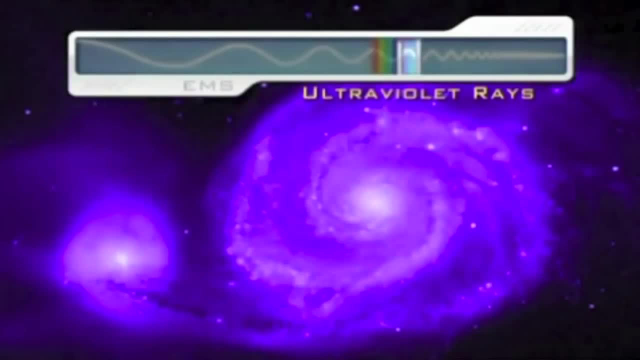 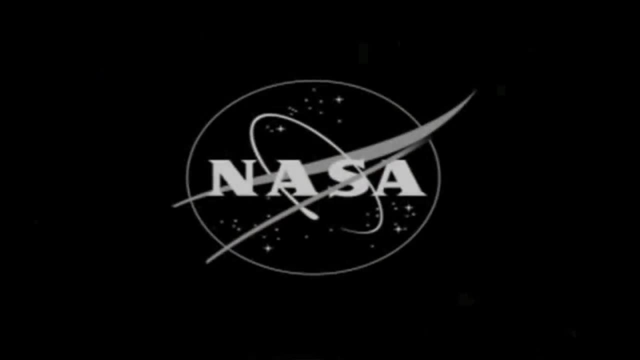 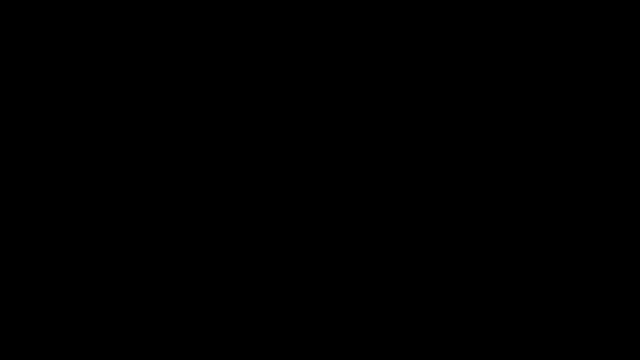 by taking advantage of the unique information contained in the different waves across the EM spectrum. So the electromagnetic spectrum includes all the types of energy flying around in the air, on Earth and in the universe. What you should have noticed from the video is that there's a variety of kinds of energy on the electromagnetic spectrum. 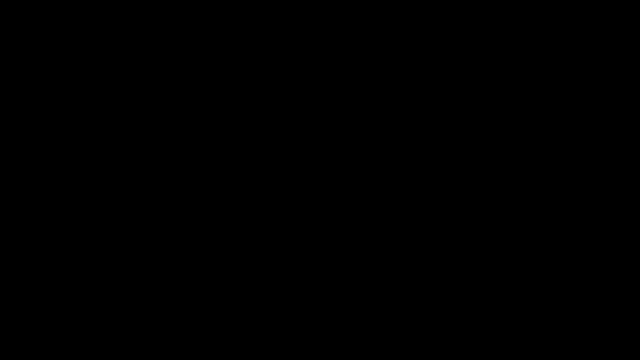 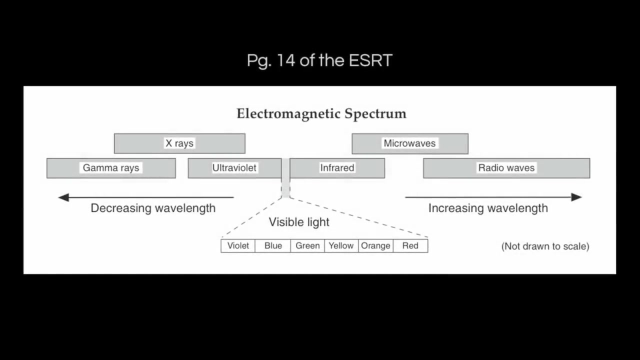 They're all different from each other based on the fact that they have a different wavelength, and that's a key idea. Fortunately for us, on page 14 of the Earth Science Reference Tables, we have a chart summarizing the types of energy found on the electromagnetic spectrum. 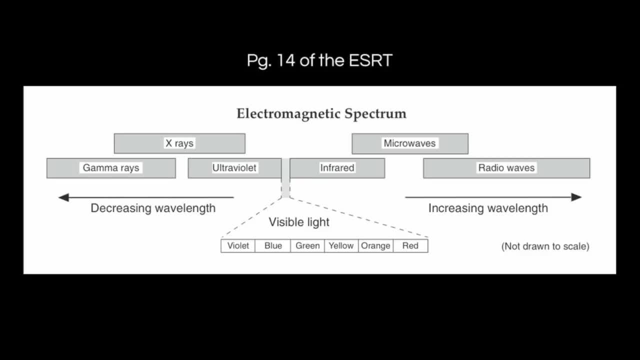 It's a very simple chart that lists the different types of energy and whether or not they have short-term effects. Let's take a look. What you'll notice is that on the far left of the chart we have the shorter wavelength energy, And you might remember from the video. 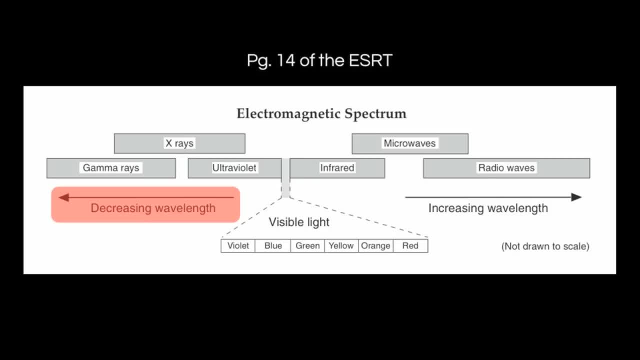 this is more energetic and therefore this is more harmful to living things. The shortest of all wavelength energy is called a gamma ray. Then we have x-rays. Yes, these are the same kind that you would get when you go to the dentist or the doctor. 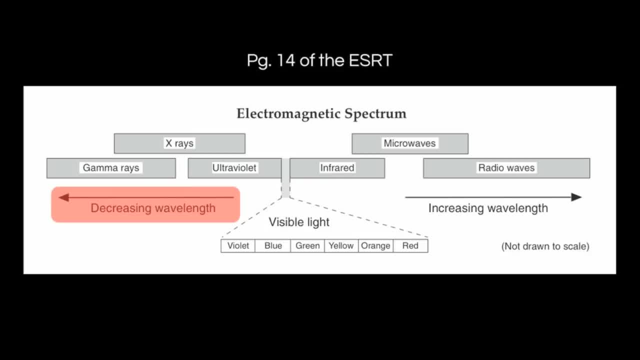 to check if you have a broken bone. It's a strong type of short wavelength energy. Then we have ultraviolet energy, And these three are generally considered the short wavelength types of energy. On the right side of the chart we have longer wavelength energy. 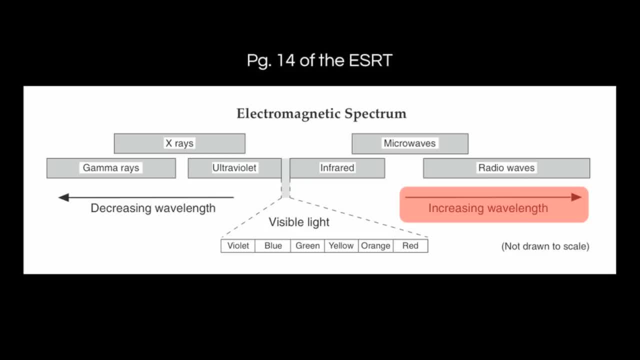 including infrared, which we feel is heat, microwave radiation and radio waves. Microwaves are what allow your cell phones to communicate with each other, while radio waves transport- you guessed it- radio signals. Now, out of all of this energy flying around, 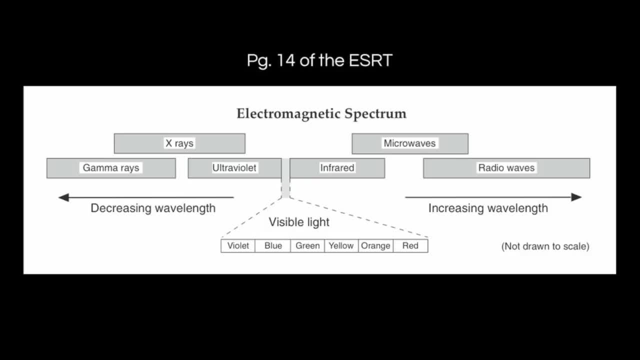 there's a very, very small band of wavelengths which humans can actually detect with their eyes, And that is called the visible light energy, or the visible light portion of the electromagnetic spectrum seen here in the center. What you'll notice is it's a very small portion. 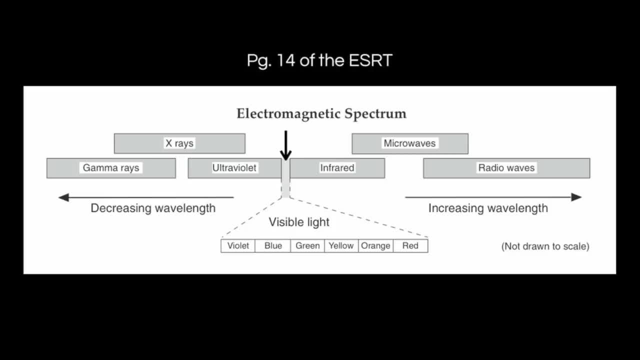 of the entire spectrum, And what that means is that, of all of the energy flying around on Earth and in space, we can only detect a very small bit of it with our eyes, But what we can detect, we can distinguish as the colors of the rainbow. 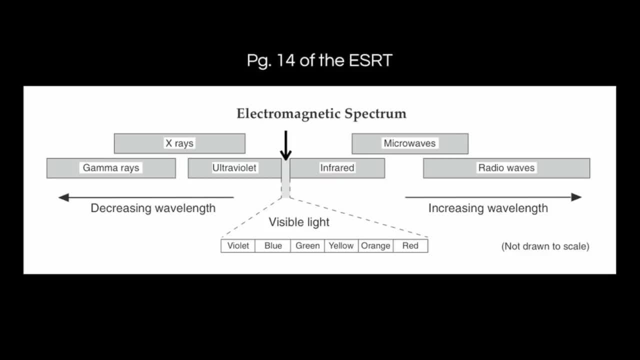 What you notice on the chart is that visible energy is broken down into the six colors of the rainbow, with the shortest wavelength on the left-hand side being the color violet. Next to violet, with a longer wavelength, is blue, then green, yellow. 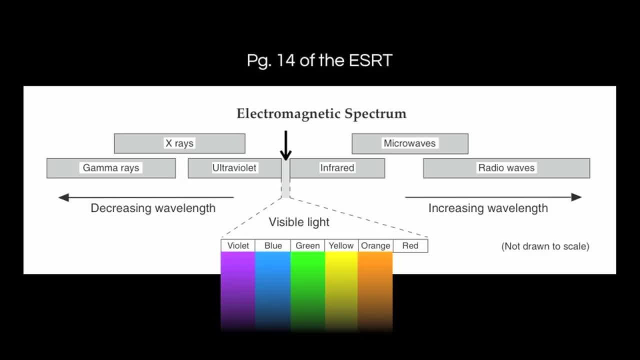 longer still would be orange, and the longest wavelength color is red. So those are the colors that make up the rainbow, and this is what allows us to detect colors in the universe and on Earth around us. What I'd also like to point out is that 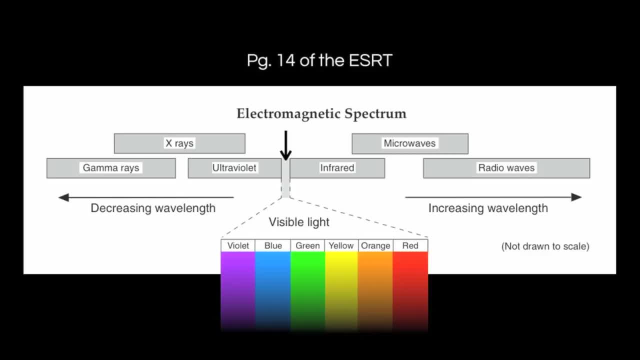 next to the color red on the chart is the next type of energy, which appropriately is called infrared. And again we can't see infrared, though we can detect it as heat. Similarly, on the left side of the visible light spectrum. 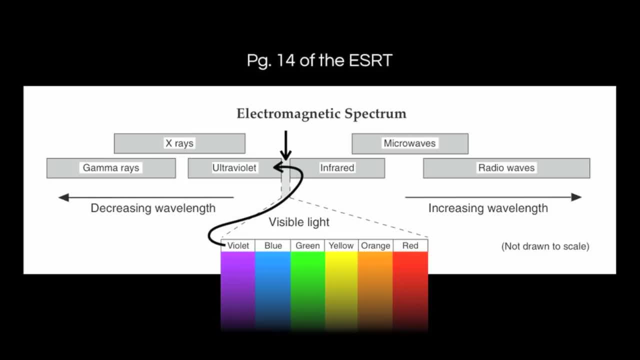 where the color violet is next to that would be found. ultraviolet. This, too, we cannot detect, though it is flying around in the Earth, emitted by the Sun. Ultraviolet is the type of energy that gives us a sunburn when we go outside in the Sun for too long. 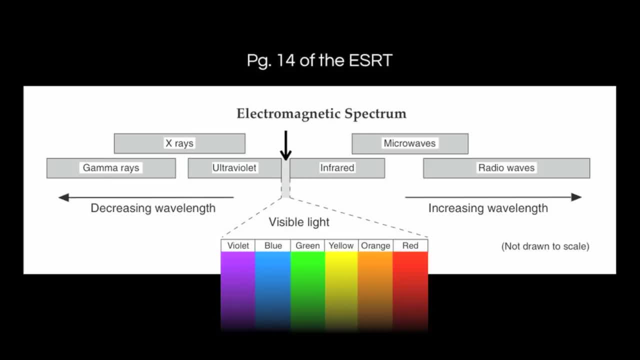 The Sun does emit primarily these three types of energy- ultraviolet, visible light and infrared- with the majority of it falling in the visible light spectrum. This is fortunate for us, because we don't want too many gamma rays or X-rays floating around. 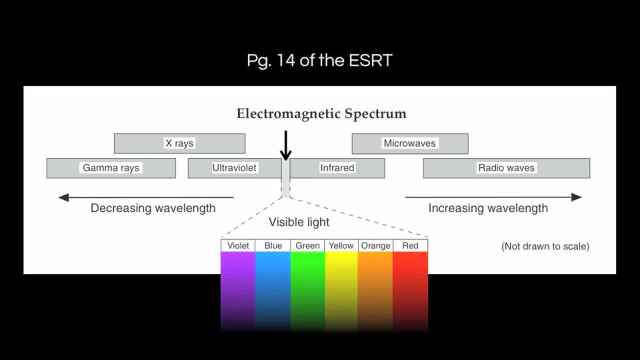 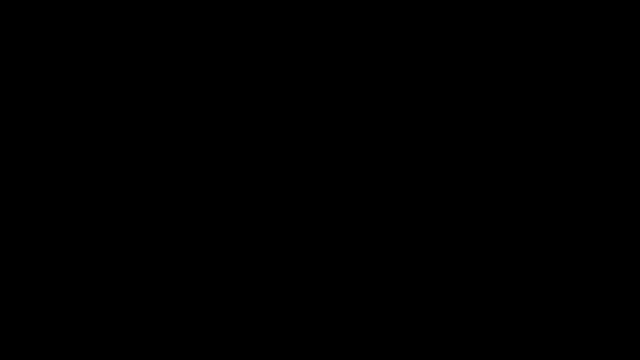 as they can harm living things. So let's imagine we took a telescope and pointed it at the Sun and collected light from the Sun and sent it through a fancy machine called a spectrometer. What we would end up with is a crazy-looking image like this: 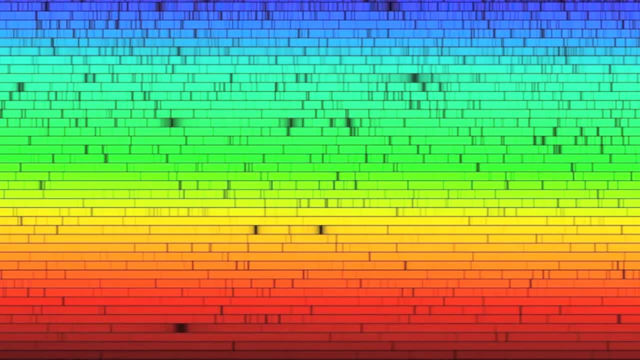 This is the visible spectrum of the Sun, And what you notice is that the visible spectrum reflects all the colors of the visible light, essentially the rainbow. But what I also want to point out are these strange-looking black lines. Think of these as the fingerprints. 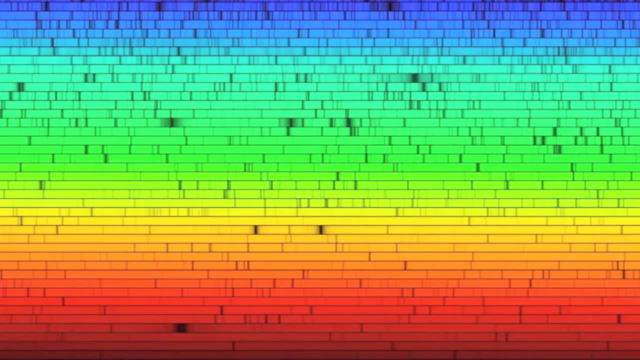 of the different elements making up the Sun. For example, the Sun is largely made of the element hydrogen, and so within these black lines is the fingerprint of the element hydrogen. Why is this important? Well, it allows us to determine the elements that make up a star or a galaxy. by just looking at the light given off from that star or galaxy. It's amazing what we can learn by looking at energy. We can learn how hot, and therefore how large, an object is. We can learn what elements it's made of. 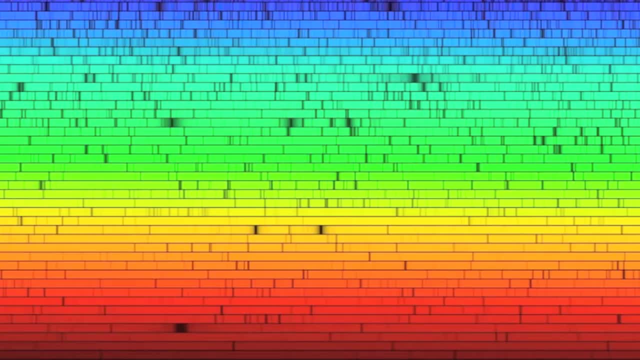 More importantly, though, we can use these spectra to determine if an object is moving. We can tell if something is moving towards us or away from us, And that would set the stage for one of the most important theories in the history of astronomy. 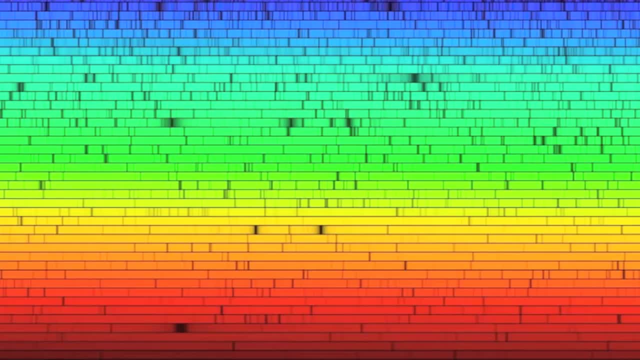 the Big Bang Theory. That's what we'll be talking about in the coming days. Thanks for listening.